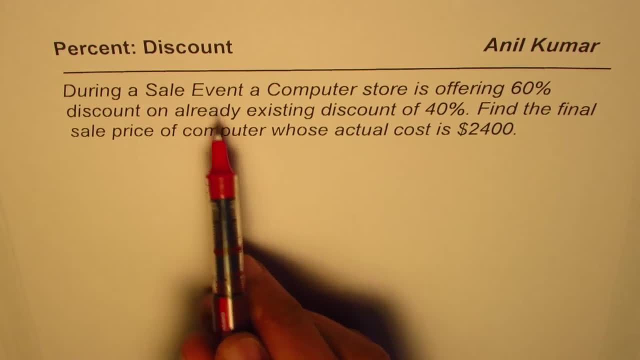 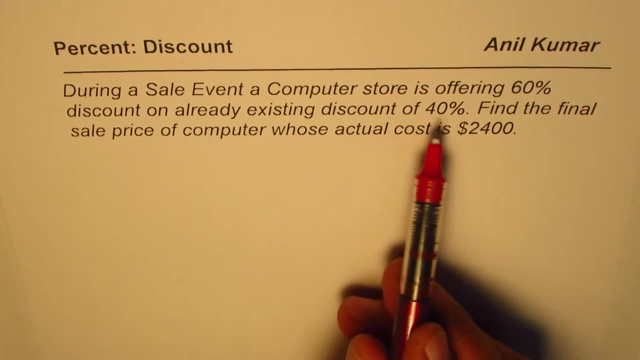 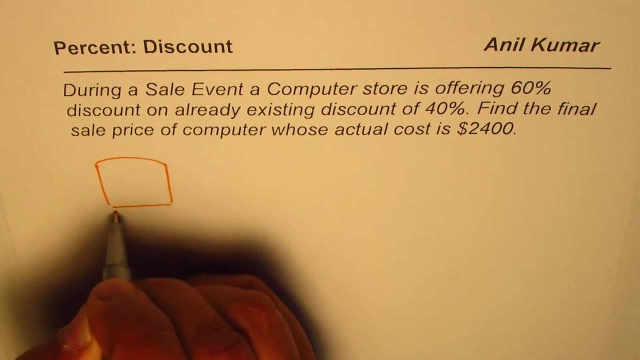 Question here is: during a sale event, a computer store is offering 60% discount on already existing discount of 40%. Find the final sale price of the computer whose actual cost is $2400.. So what we are given here is kind of: let us say: we have a computer here, right, So we have this computer. Okay, now what are we given here is that this Computer's original price is $2400.. Now it is on sale. So it says: during a sales event, a computer store is offering 60% discount on already existing discount of 40%. So it's minus 40%, And then, based on this, we have a further discount of 60%, right? So that is the case, And we have to now find. 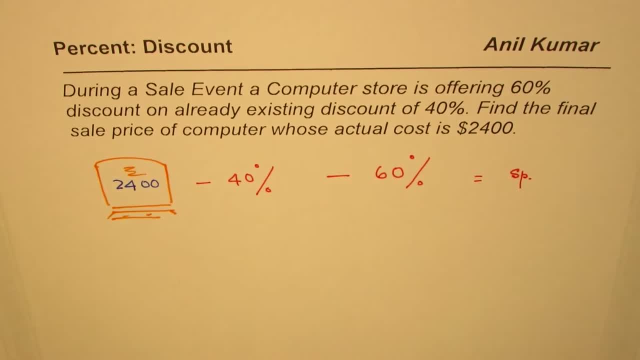 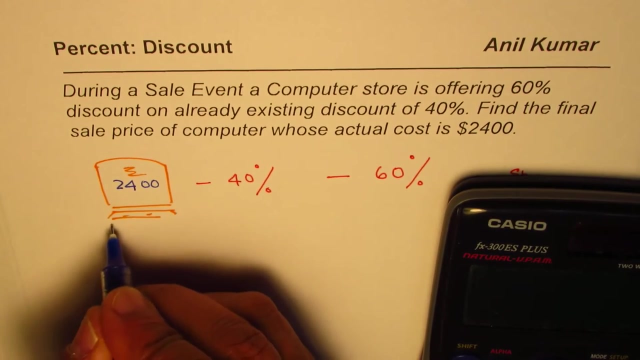 What is the final selling price correct? So that is the question. You can actually pause the video, answer the question and then look into my suggestion. Now, 40% of $2400 is how much? Let's find that. So let's find 40% of $2400.. So 40% of $2400 is 0.40 times $2400. 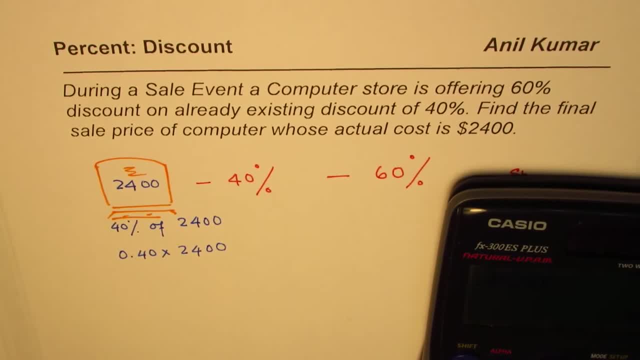 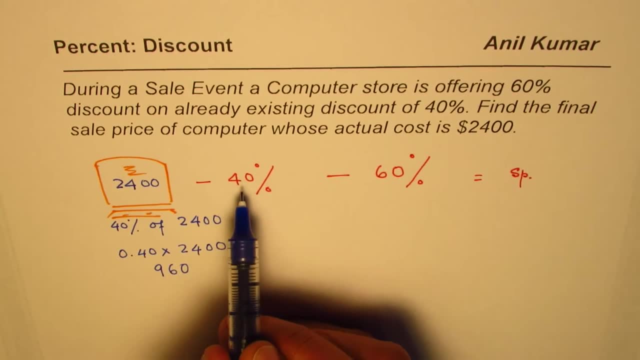 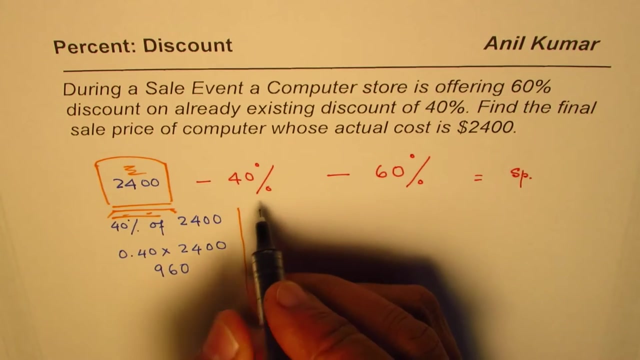 0.40 times $2400 is $960, right, It is $960.. So once you put that discount, then the price after discount will be how much. Let's write it down. So let's write down here Selling price one that is after 40% discount. it should be $2400. take away $960, right. 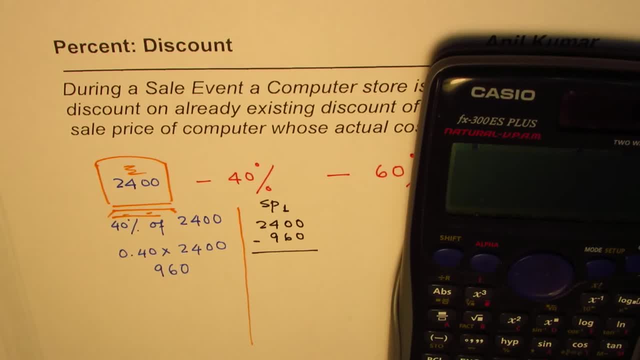 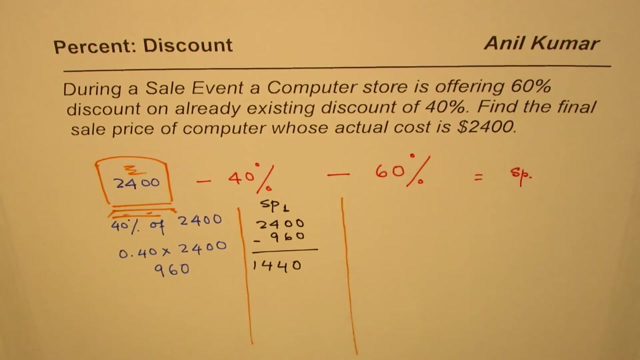 So that is the cost of 2400. take away discount of 960, so that gives us a value of 1440 dollars. is that okay? now we are given further discount of 60 percent on this price. this is important to understand, right. it is not all. this is 100 percent. we are not getting 100 percent on 2400. that is zero dollars. 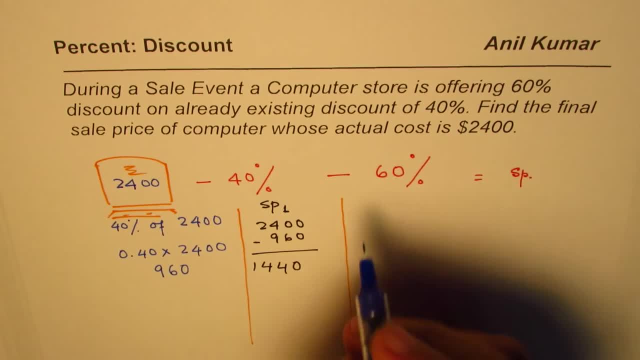 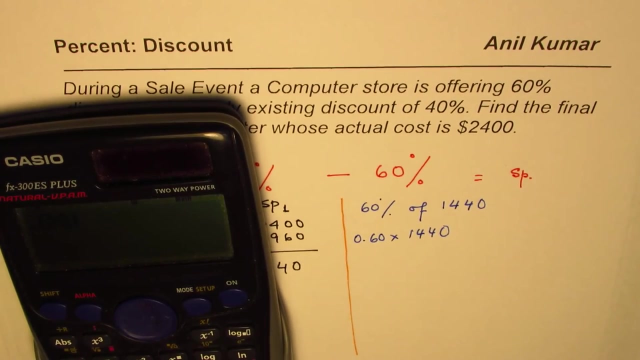 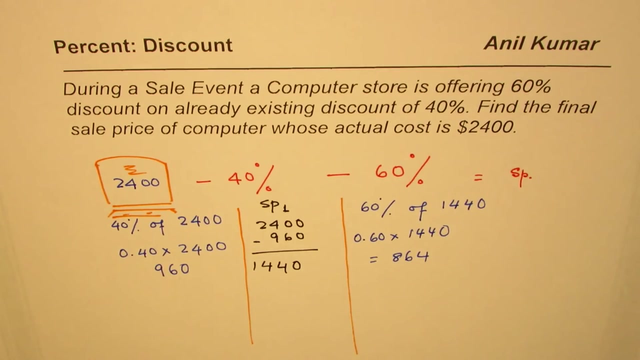 to pay correct, okay? so what is 60 percent of? let's calculate 60 percent of 1440, that is 0.60 times 1440. okay, let's find it out. so it is 0.6 times 1440 equals to 864. so if 864 is the discount,